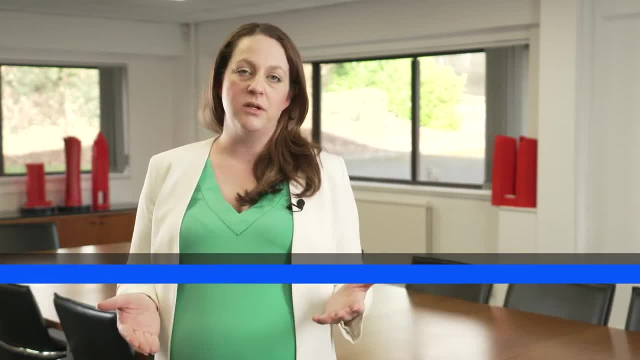 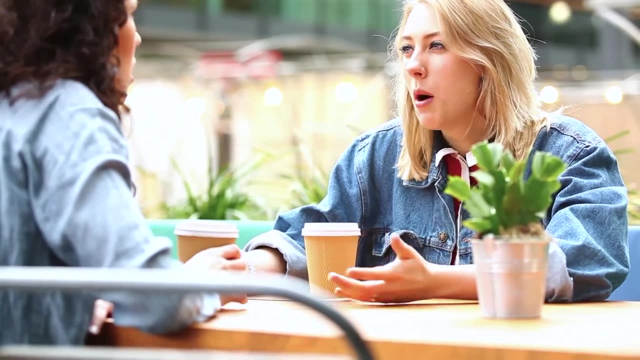 environment, and this varies depending on what I'm doing as a human. So if I'm sat out in London having my coffee, and I'll be really sensitive to air movement. if it's cold and the air is moving across my skin, that can make me feel quite uncomfortable. However, 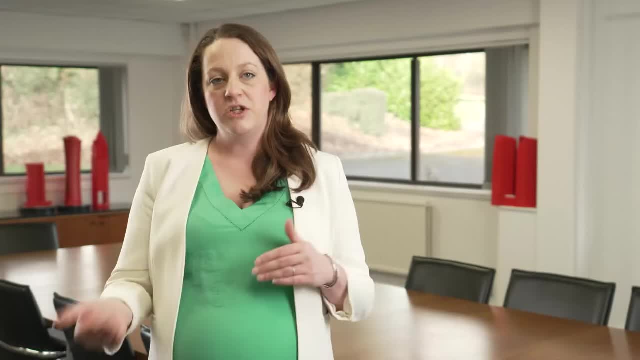 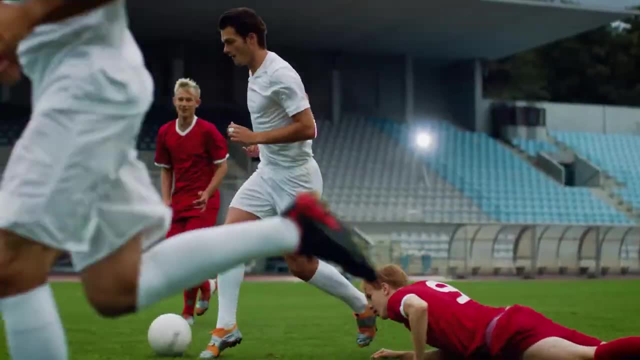 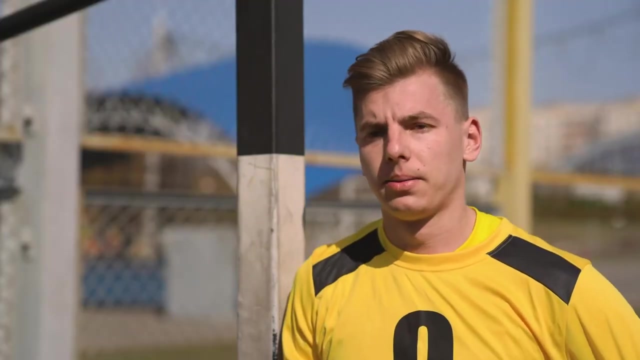 if I have direct sun on my face then that will warm me up. Switching for a moment: if we think about an elite sports person, that person might need to run as hard as they can for many, many minutes. In that case, I would be really interested in understanding how much moisture is already in the air. the 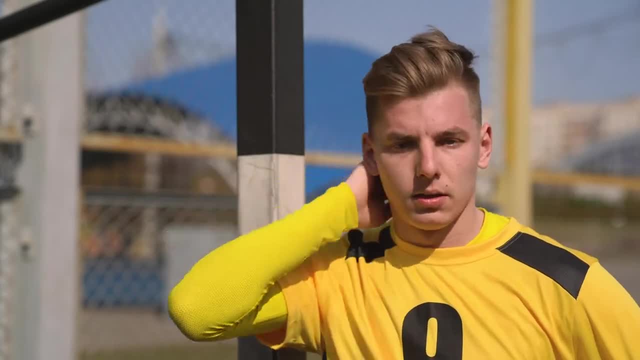 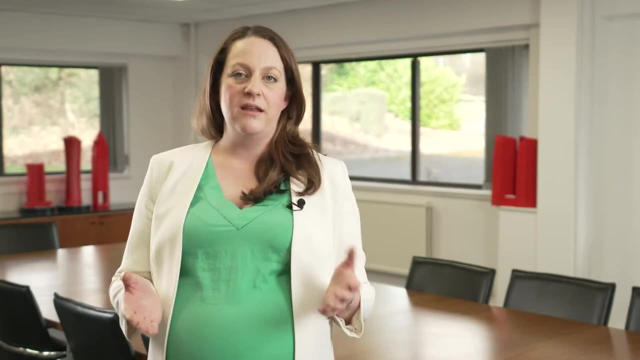 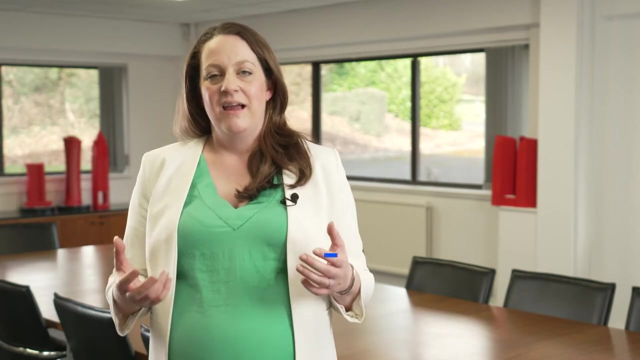 humidity in that environment and therefore the ability of that elite sports person to evaporate sweat that they're producing to regulate their temperature. So, with my understanding of the climatic environment and the physical response of me as a human, the next thing I need to consider is my expectation. 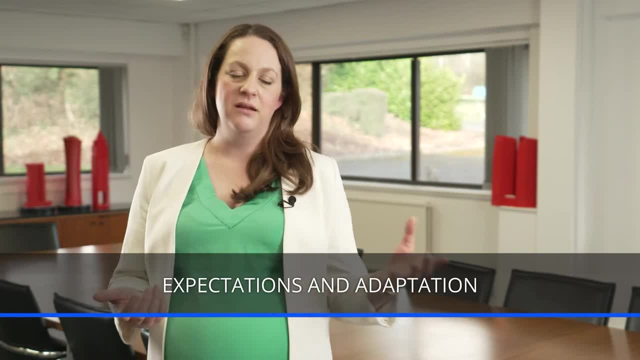 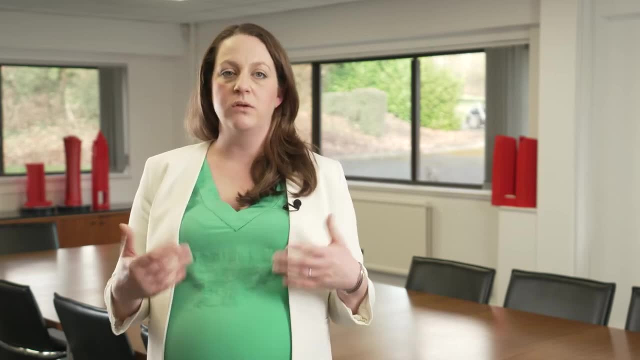 and my ability to adapt to my environment. So again, in London we have a very variable climate. I will always look at the weather forecast before I go outside and if it's going to be cold and dry and I want to sit out, I'll put on a thick coat, a scarf and a hat and I'll go out and I'll expect to. 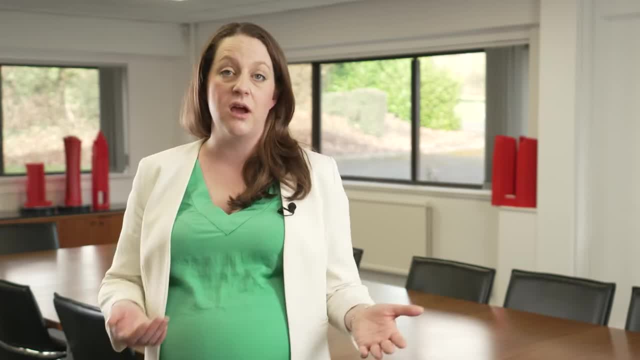 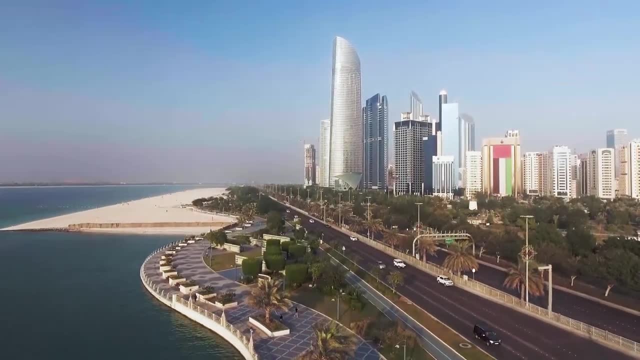 be in a comfortable environment to have my coffee, enjoy the sunshine, and I'm not concerned about the cold weather. If, however, I want to walk along the Corniche in Abu Dhabi here, I don't expect to be able to do that in the middle of the day in July, because it is just too hot. 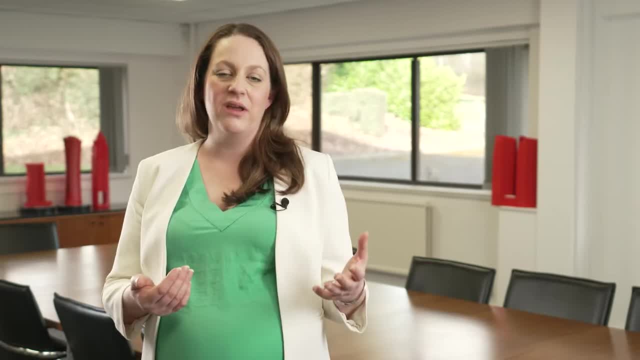 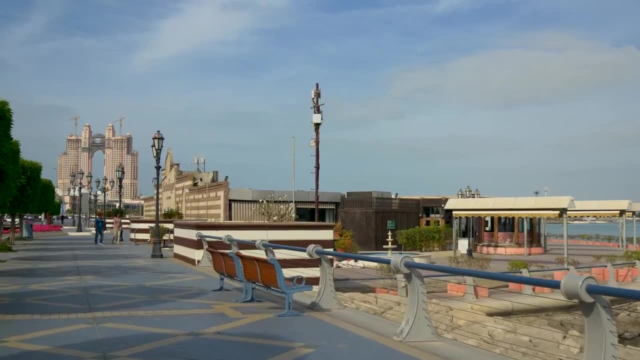 However, with the right design, I can do that same walk in the evening in the summer or in the middle of the day in winter, by provision of shade and ensuring I'm getting those sea breezes that cool me down. The final piece of the puzzle is: how do we measure success? What does good look like? 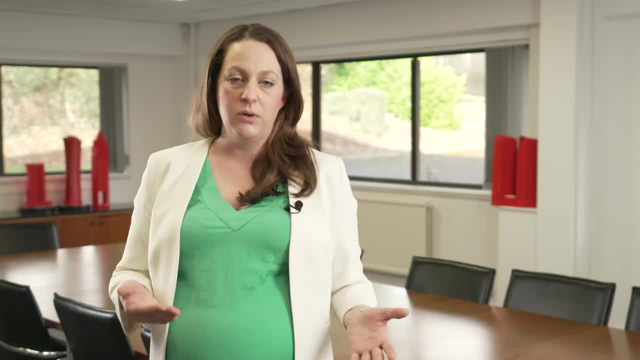 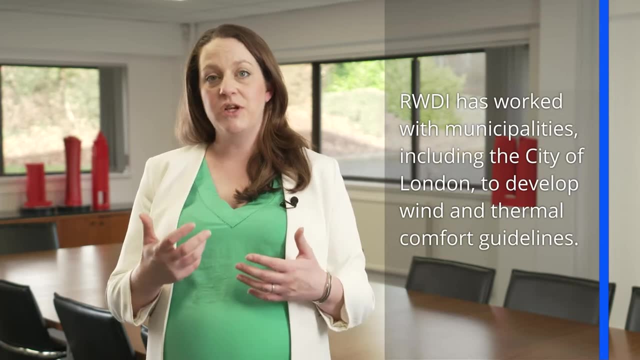 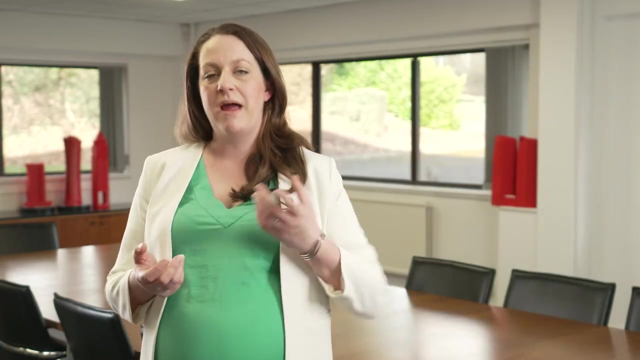 And again, this varies depending on what activity we're looking at and where we are in the world. There are areas, such as London, where we have thermal comfort measures which are actually required as part of our planning or our permitting process, And there are other parts of the world where we would choose the appropriate metric which combines those variables that I've just talked about, to give us a measure of pass or fail, or success or failure.